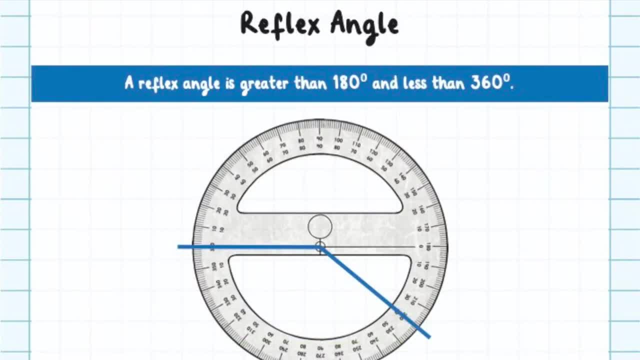 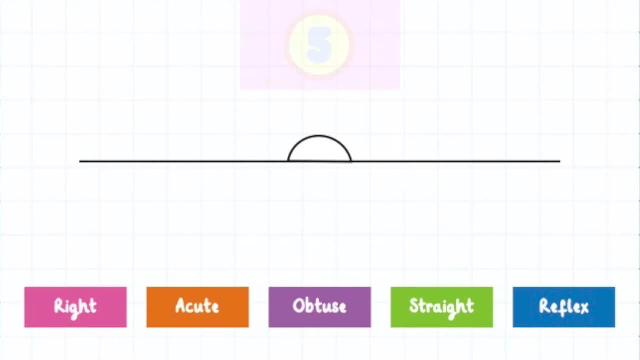 A reflex angle is greater than 180 degrees and less than 360 degrees. Quick quiz. What kind of angle is this? This is a straight angle. What kind of angle is this? This is an obtuse angle. What kind of angle is this? 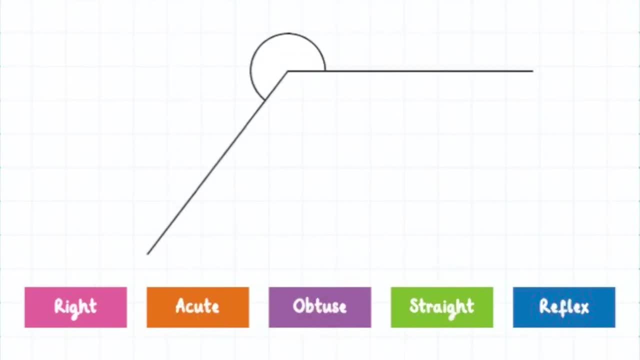 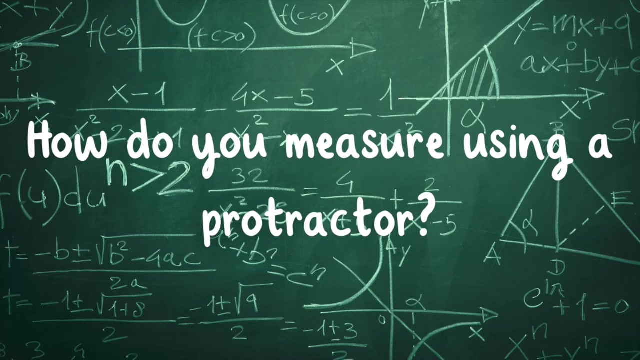 This is a right angle. What kind of angle is this? This is a reflex angle. What kind of angle is this of angle? is this? This is an acute angle. How do you measure using a protractor? Although it may seem tricky to understand at first, we promise. 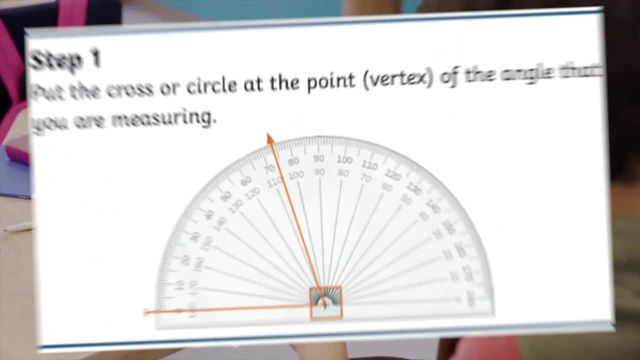 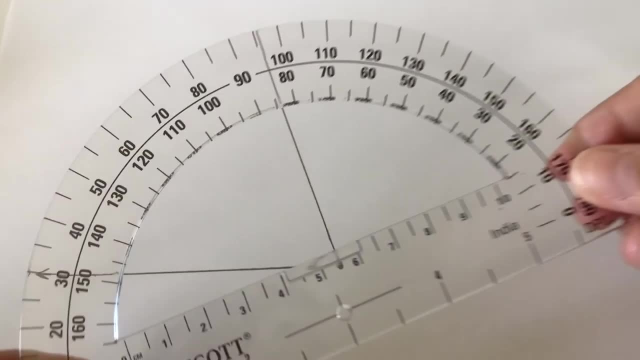 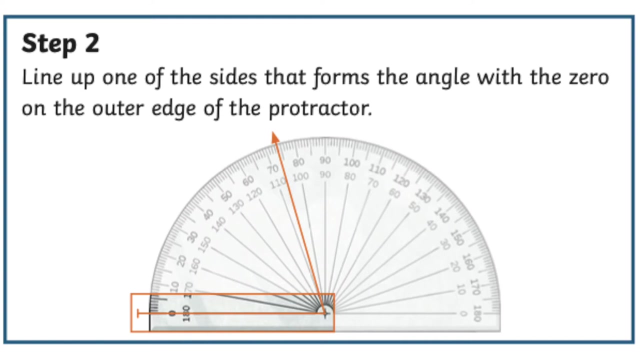 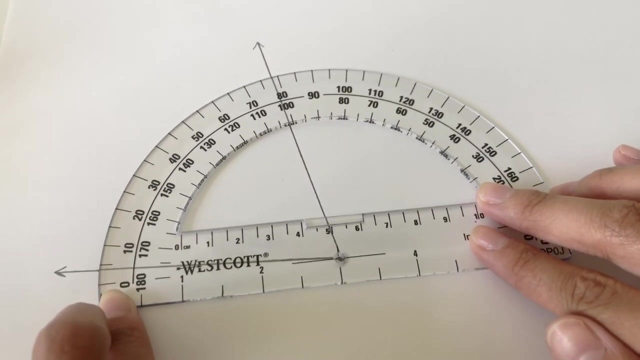 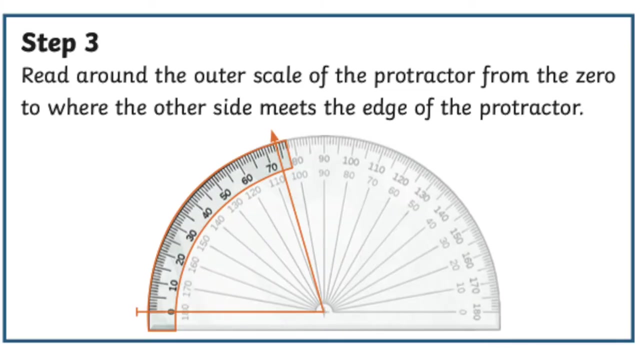 protractors are not difficult to use. First put the cross or circle at the vertex of the angle that you are measuring. Next, line up one of the sides that forms the angle, with the zero on the outer edge of the protractor. Then read around the outer scale of the protractor, from the zero to where the 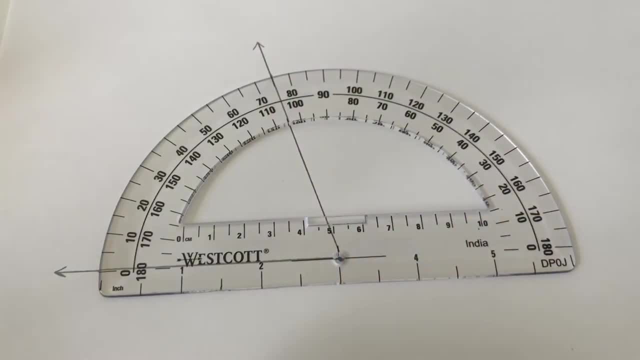 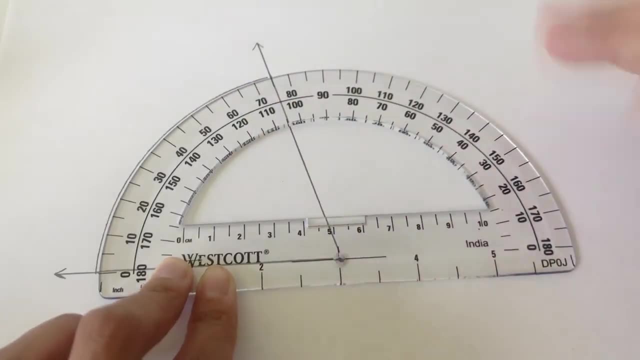 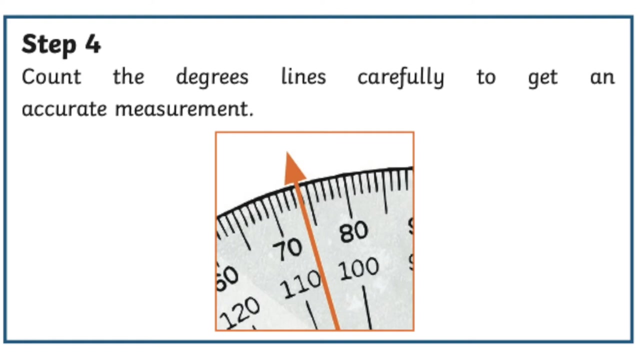 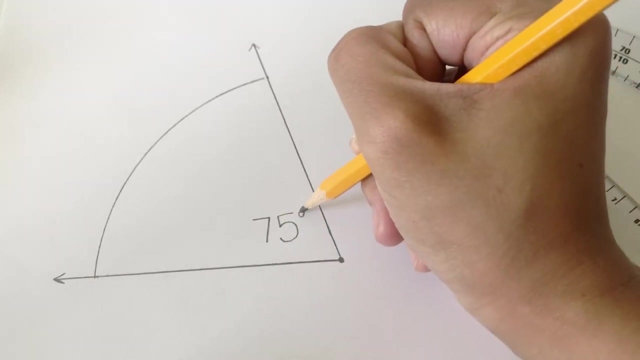 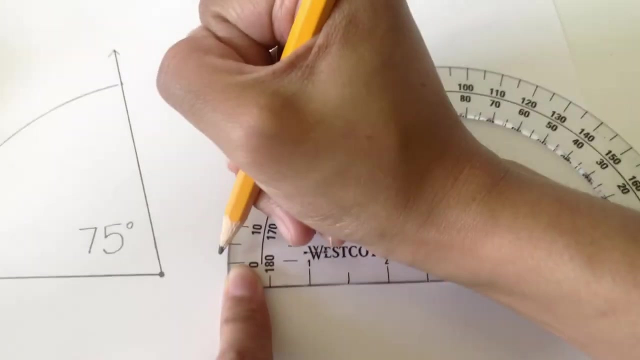 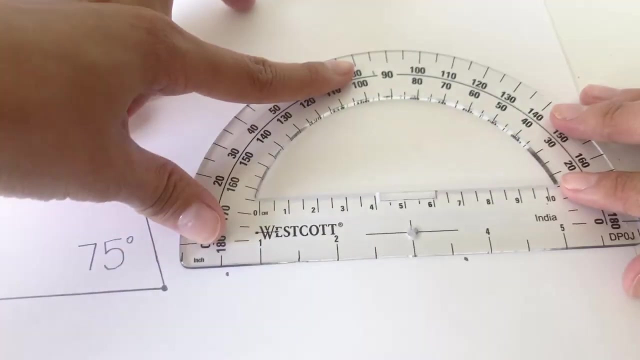 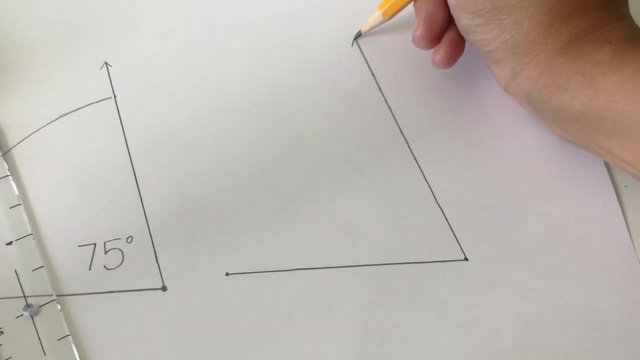 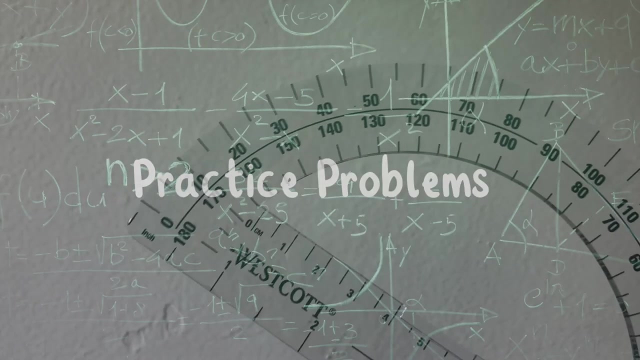 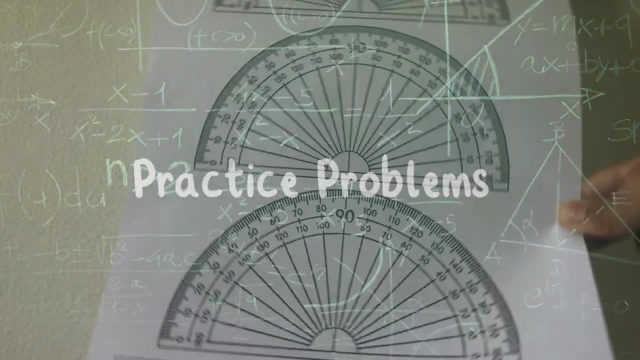 other side meets the edge of the protractor. Last, count the degree lines carefully to get an accurate measurement. Practice problems: Use a protractor to draw each of these angles. If you don't have a protractor at home, give this printable protractor a try. 45 degrees. 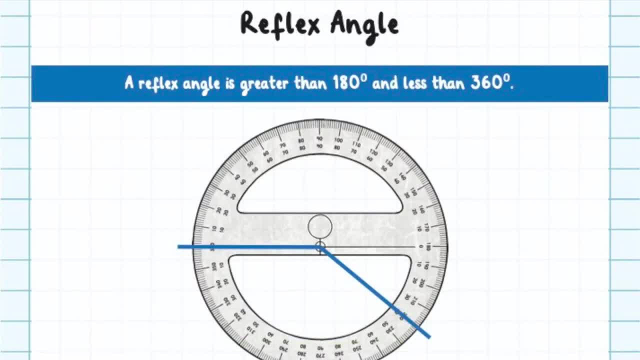 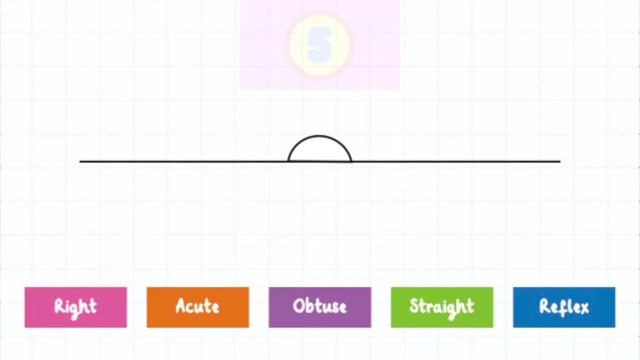 A reflex angle is greater than 180 degrees and less than 360 degrees. Quick quiz. What kind of angle is this? This is a straight angle. What kind of angle is this? This is an obtuse angle. What kind of angle is this? 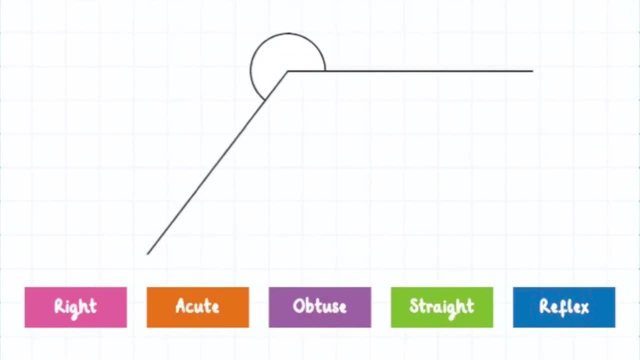 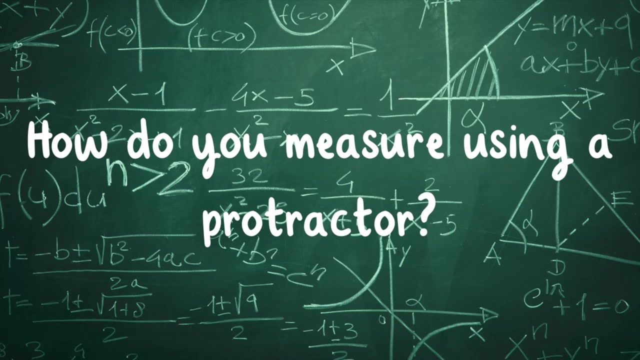 This is a right angle. What kind of angle is this? This is a reflex angle angle. What kind of angle is this? This is an acute angle. How do you measure using a protractor? Although it may seem tricky to understand at first, we promise protractors. 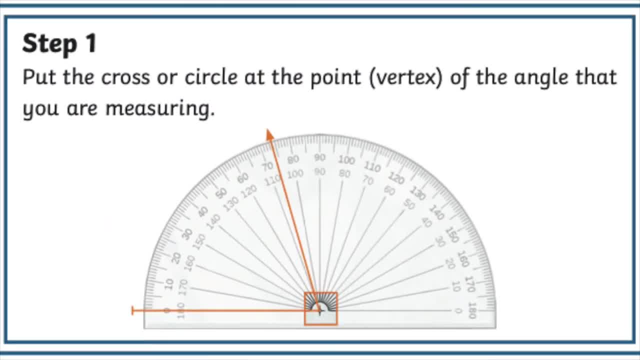 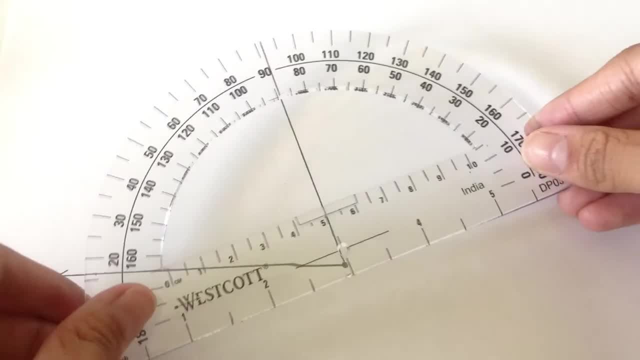 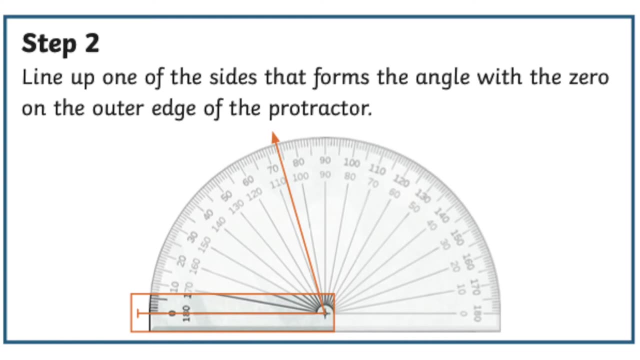 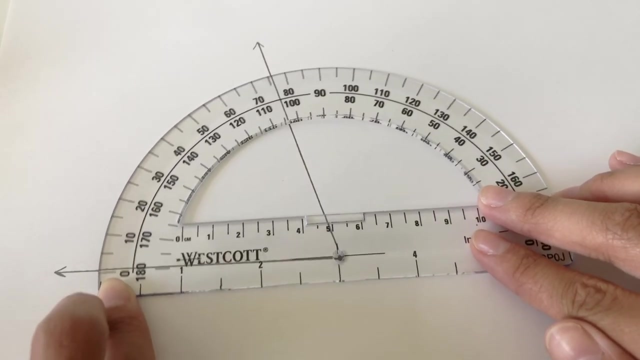 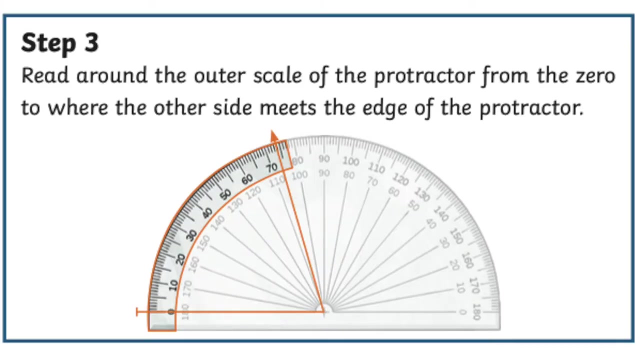 are not difficult to use. First put the cross or circle at the vertex of the angle that you are measuring. Next, line up one of the sides that forms the angle, with the zero on the outer edge of the protractor. Then read around the outer scale of the protractor from: 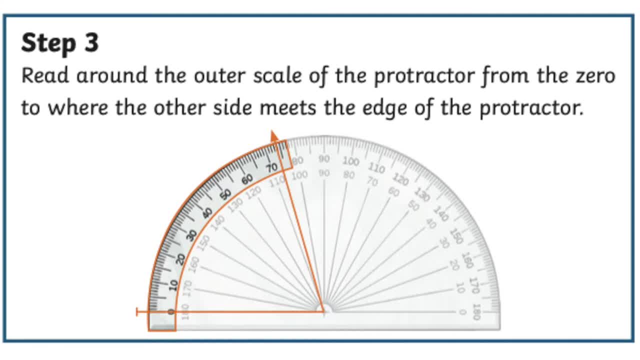 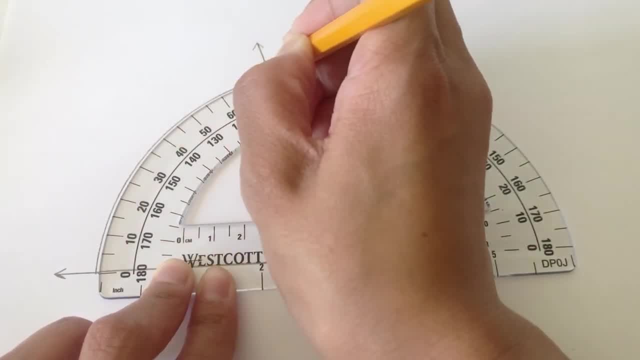 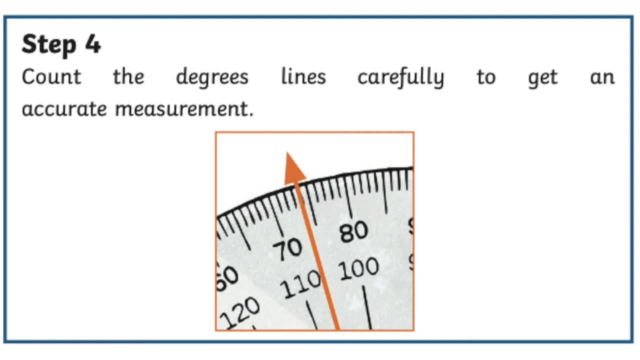 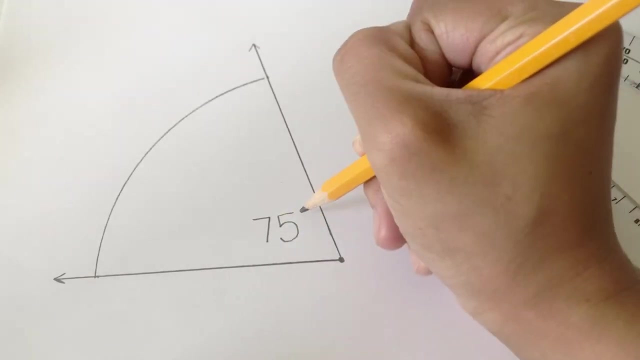 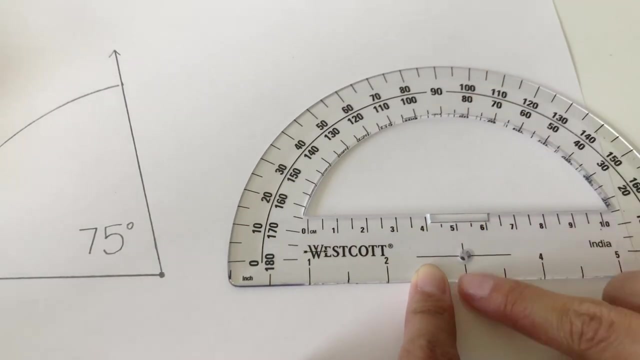 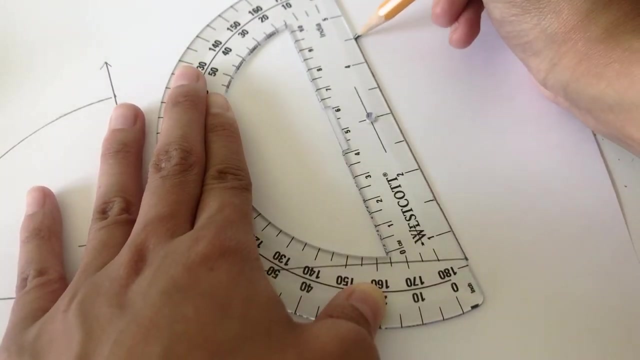 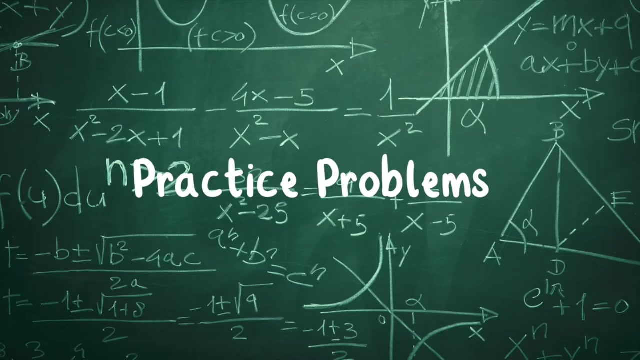 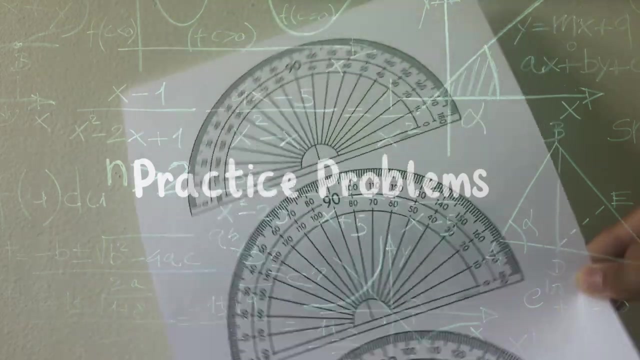 the zero to where the other side meets the edge of the protractor. Last, count the degree lines carefully to get an accurate measurement. Practice problems: Use a protractor to draw each of these angles. If you don't have a protractor at home, give this printable protractor a try. 45 degrees.